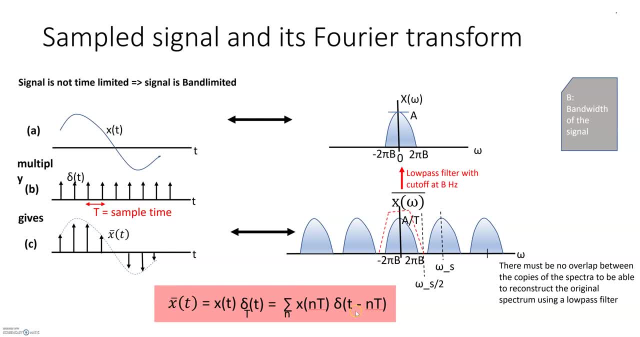 Now let's focus on this equation, which we didn't really discuss in the last slide. So this signal, the sampled signal, is essentially the original signal x of t multiplied with the impulse train. So that's pretty much what it is. 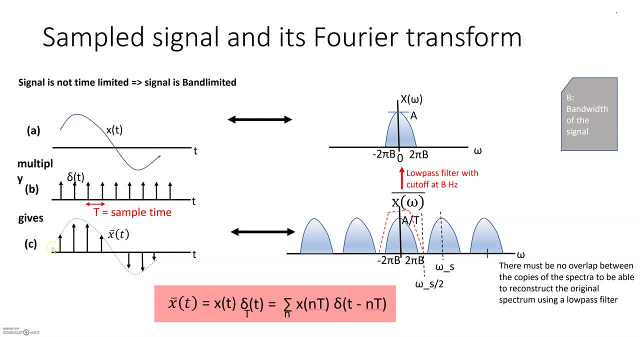 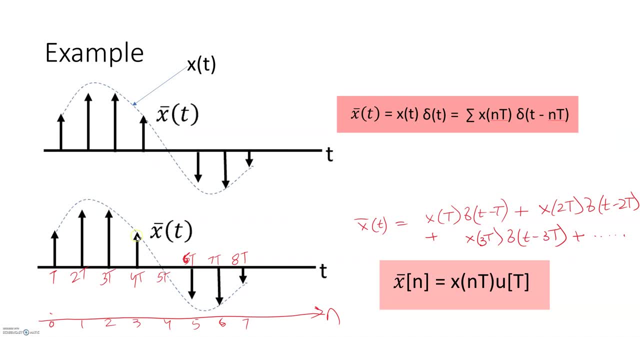 We can also rewrite this signal as the summation of individual samples. What that means is that: So let's look at this figure in the bottom, So this, these are our different samples. So let's say: this is a sample that we got at, this is our first sample. 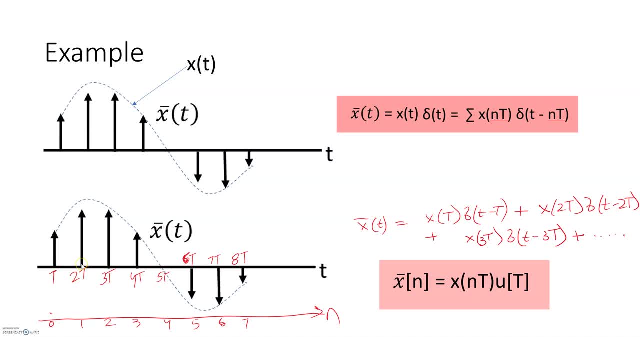 Then, after the fixed interval t, this is our second sample, This is our third sample. So these are just the samples at fixed time intervals. So this is how we can write that when on the x-axis you have time, We can also define this signal by putting it on the axis that gives us the number of samples. 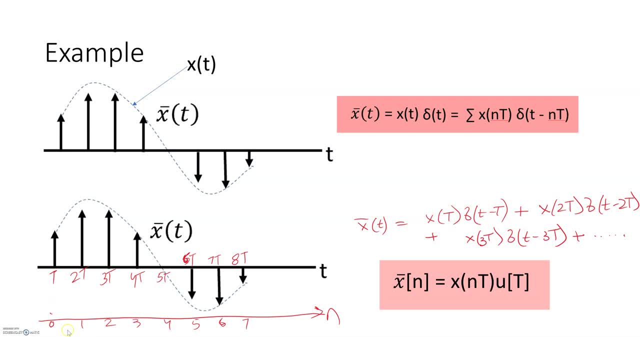 So, instead of saying time here now, these are individual samples. This is the first sample, second sample, third sample, fourth sample, and so on. Therefore, we can rewrite this equation, that is the definition of the sampled signal, as x, n of t times u of t. 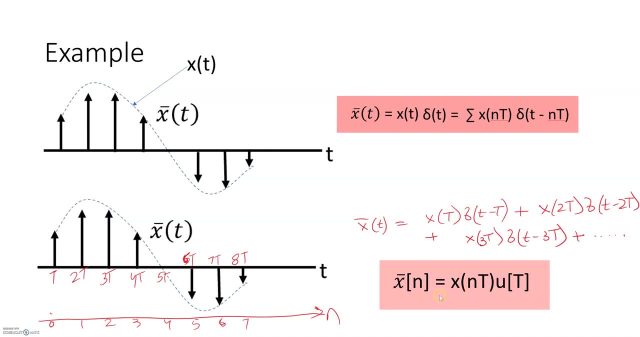 So we can write this equation as x, n of t, times u of t, times u of t. What that really means is that the value of the sample, the value of the sample at the value of the nth sample of the sampled signal, is really the value of the original signal, calculated at time n of t. 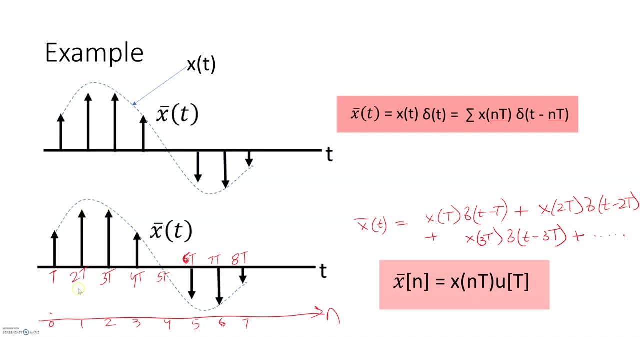 So let's- I think this is clear from this figure here. So let's say We are talking about the second sample which is here, So the value of the second sample is going to be equal to the original signal calculated at time 2t. 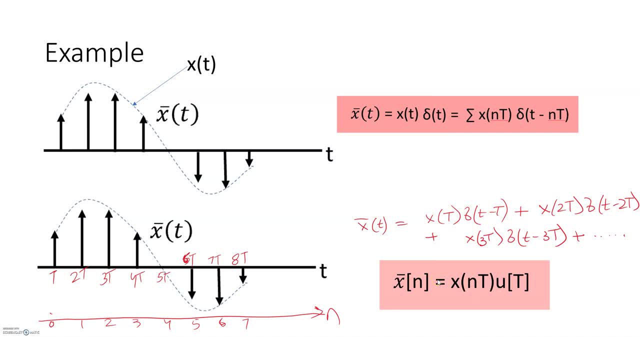 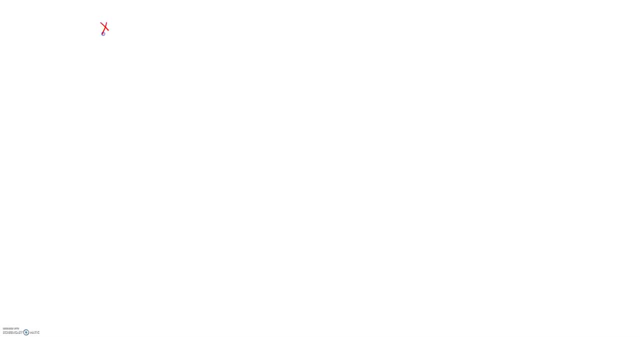 So that's really what this equation is. Let's do an example to understand it further. So let's say we are given a continuous time analog signal That is defined by 2e negative of pi, t times u of t, And we want to convert this signal to analog discrete time signal. 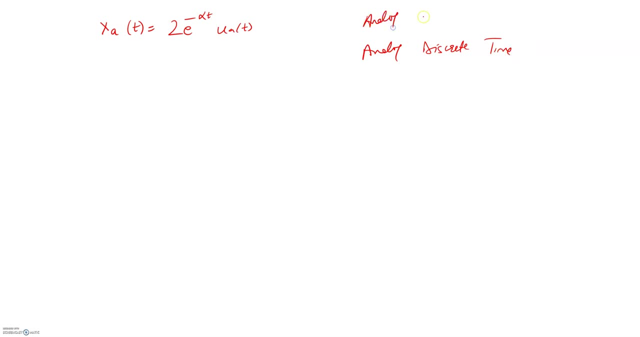 We want to convert from analog continuous time to discrete time And we are given a sampling interval as 0.17.. So what we would do is we would take this original signal x of a t and then pass that into a sampler With time interval defined as 0.1 second. 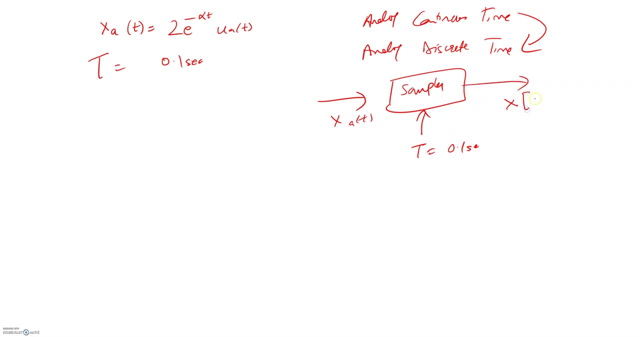 And what we should get is a digital- Sorry, Analog- discrete time signal. So how do we get this signal? In the previous slide we saw that the way we do that is basically: we find the samples, individual samples of the discrete time signal, by just finding the value of individual sample. 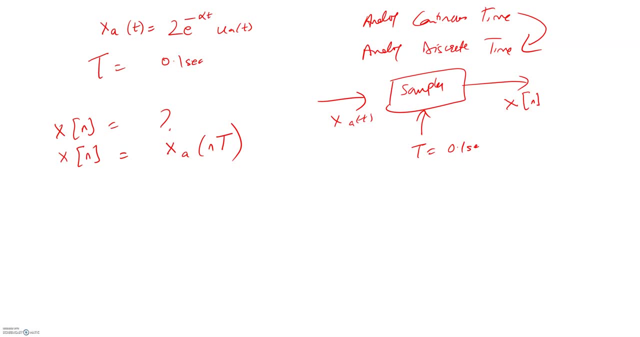 By just putting in N of t. N is the which sample into the original signal here. So if we do the math, what we get is 2e of pi, t So t. we are going to put n of t. 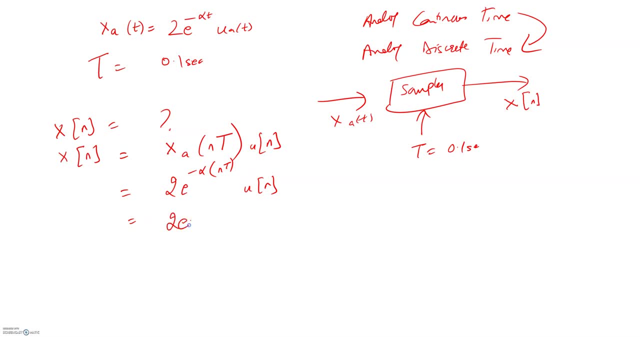 u, And then we can rewrite this 2e negative of pi t times n, n, And then, to make our life a little simpler, we will just say that a is equal to n of t. Then we get 2a to the power of n. 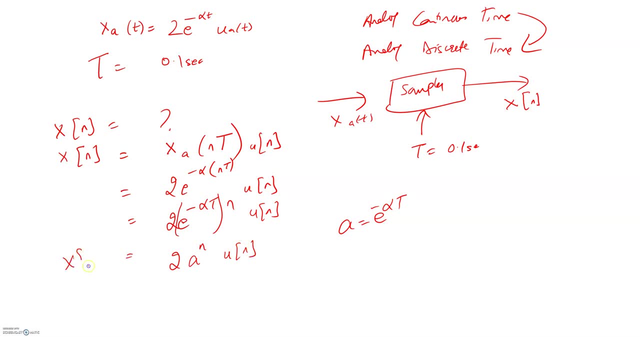 u of n. So this is the. This is how we convert from the analog to digital. I'm sorry. This is how we convert from the analog continuous time To analog discrete time. And then, if you want to find the individual samples, we really would only need to put the value of the sample: first sample, second sample, and so on. 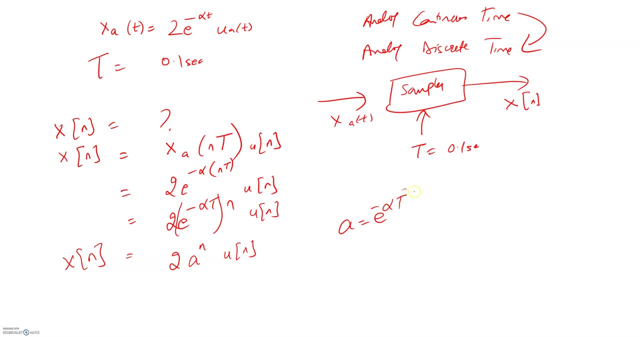 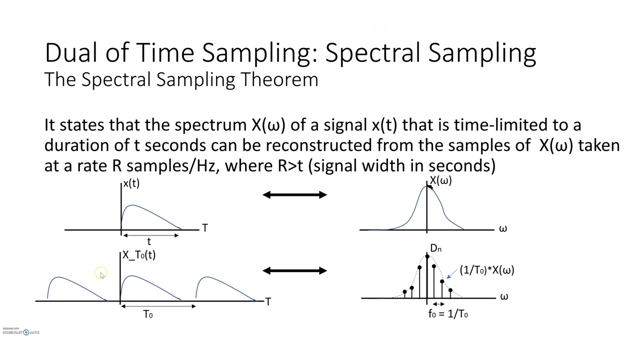 And then we have the time defined And then we will use that information to find the actual values. That's an example to do it by Now. one other thing that was not covered in the previous video Was that all we have discussed so far was the sampling in the time domain, but we can also sample in the frequency domain. 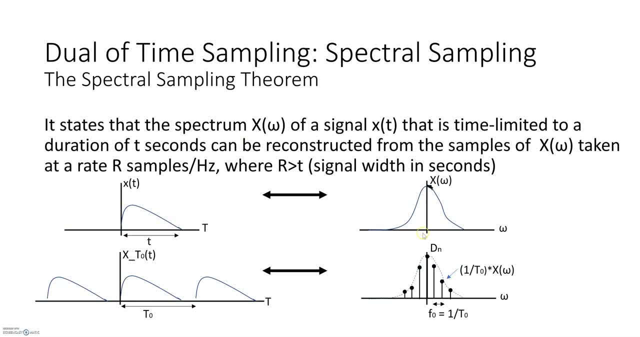 So here, instead of sampling in the time domain, we sample the spectrum just like it's shown in the diagram here, And then we have a dual of the time sampling theorem. It's called spectrum spectral sampling. sampling will not go into the details, but I just wanted to put this out there in case. 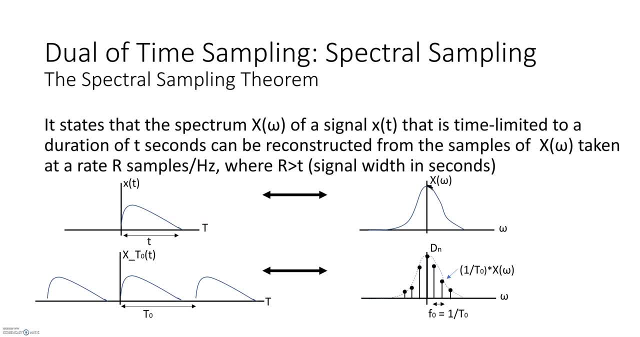 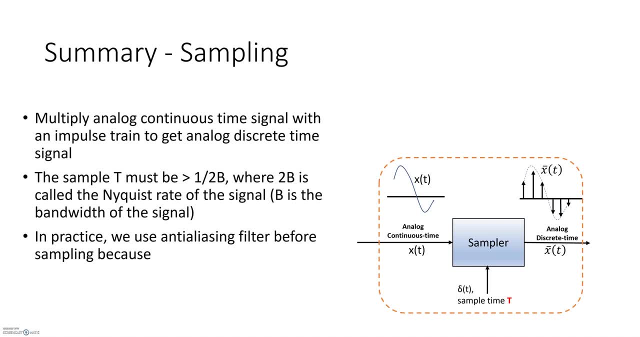 In case you come across it anytime. So this is what it is. With that we will finish the sampling portion of it. So what we have discussed in these two slides is that if they're given the analog continuous time signal, then we pass that through a sampler. 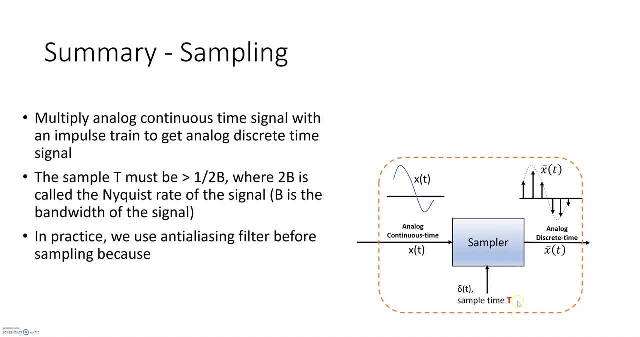 And with the sample time that we need to figure out, which really is that we should sample at a rate greater than the Nyquist rate, And then what we get is the analog discrete time signal. And then one other thing that we learned was that in practice we have a filter called anti-aliasing filter, that we pass our original signal through first before we start sampling. 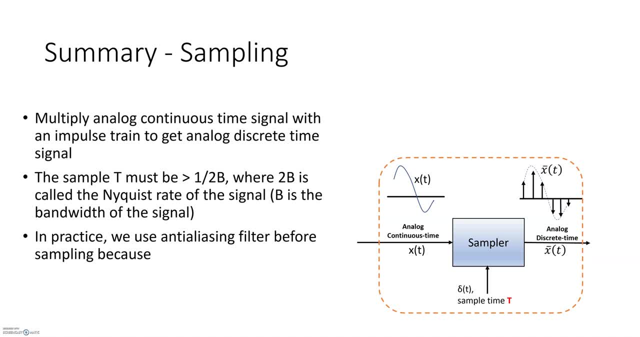 So that's it about sampling. In the next video we're going to discuss the process Of converting this analog discrete time signal to digital signal through a process called A to D conversion. So if you're interested, I'll see you in the next video. Thank you Bye.